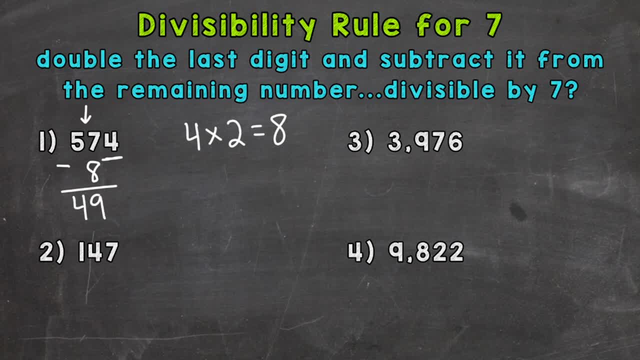 That gives us 49.. So we take a look at that remaining number there- 49, and see if it is divisible by 7.. If so, the original number is divisible by 7.. So can we do 49 divided by 7 and get an answer without a remainder. 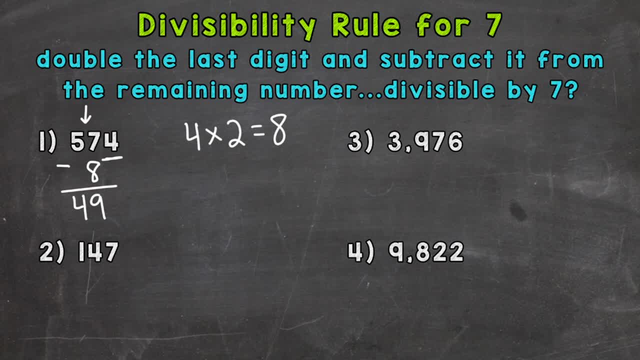 Yes, 49 divided by 7 is 7.. So 49 is divisible by 7.. Therefore, our original number- 574, is divisible by 7.. Let's take a look at number 2, where we have 147.. 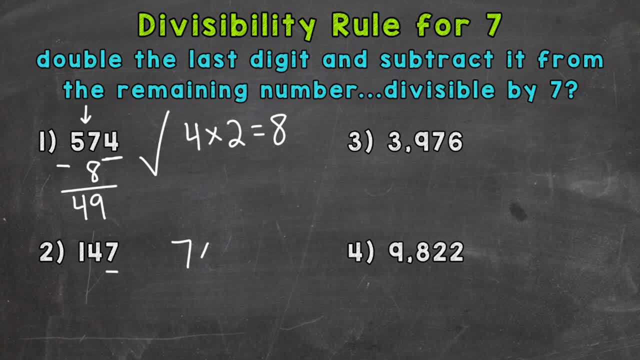 The last digit is 7.. Let's double it, So 7 times 2 equals 14.. Our remaining number is 14 here. So 14 minus 14 gives us 0.. Remember: 0 is divisible by any number. 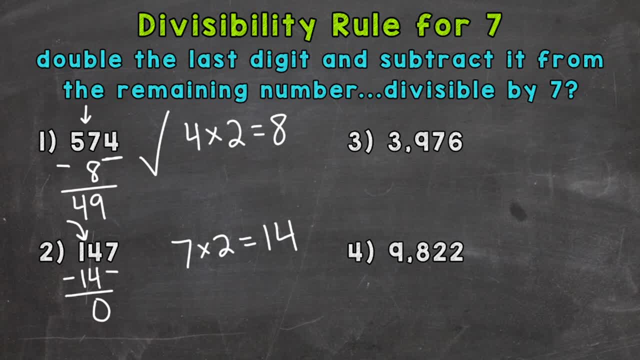 Therefore, 0 is divisible by 7.. That means our original number 147, is divisible by 7.. On to number 3,, we have 3,976.. Our last digit here is a 6.. So let's double it. 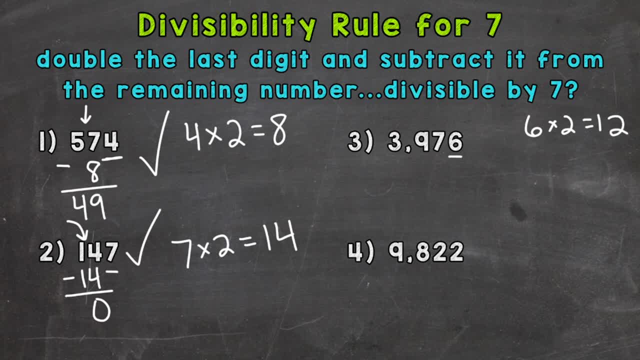 6 times 2 gives us 12.. Our remaining number is 7.. So our remaining number is 397.. So we need to do 397 minus 12.. So 7 minus 2 is 5.. 9 minus 1 is 8.. 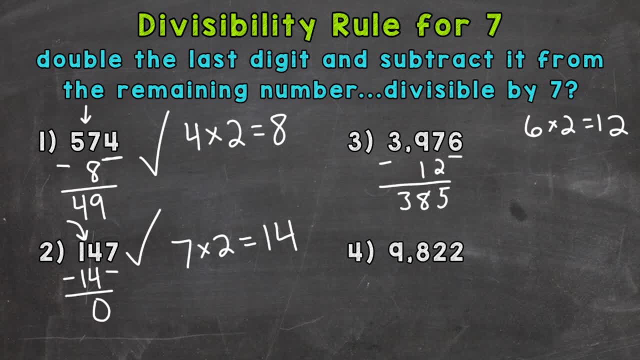 Bring down our 3.. 3 minus 0 is 3.. 385 is still kind of a large number there in value, a three-digit number. So we're going to repeat our steps actually. So what we're going to do, let's take a look at our last digit. 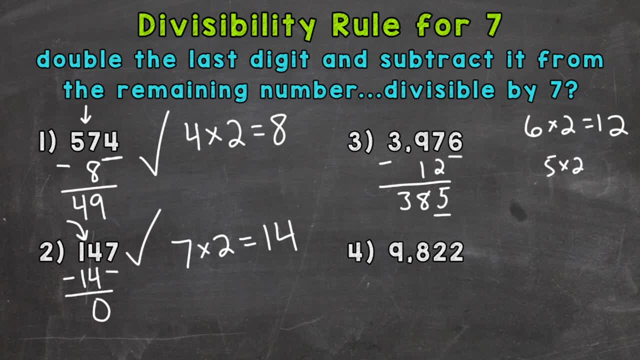 5 and double it. So we know 5 times 2 equals 10.. So we can do 38 minus that 10. And that gives us a remaining number of 28.. That's much easier to work with than 385.. 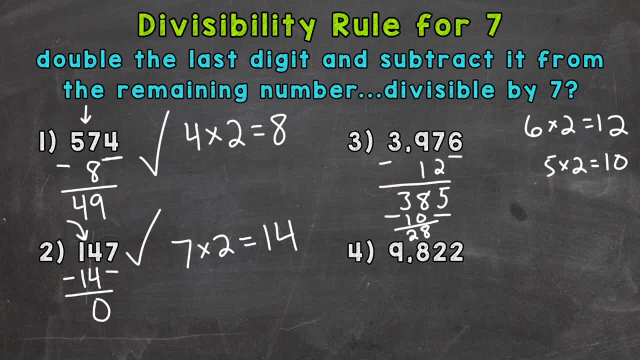 Again. we just repeated the steps to give us a more manageable number to work with. So is 28 divisible by 7?? Can we do 28 divided by 7 and get an answer without a remainder? Yes, 28 divided by 7 is 4..